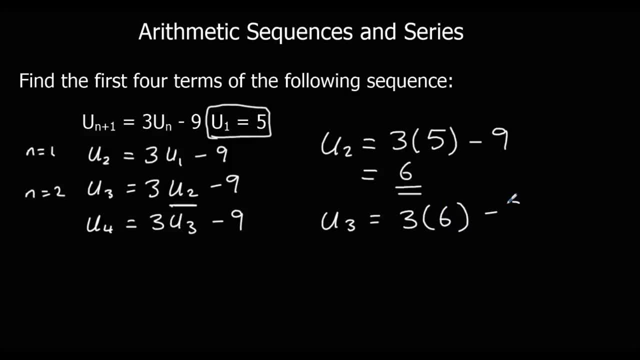 is three lots of six. take away nine, So 18,. take away nine is nine, and so on. So the fourth term is going to be: three lots of nine. take away nine, 27, take away nine is 18.. And we could keep. 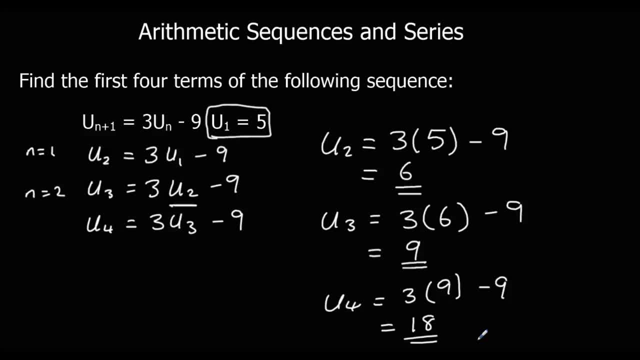 progressing like that. So in order to find the 100th term, I'd have to do three times the 99th term, take away nine and so on. Okay, so here's three questions. Pause the video and give them a go. So just substitute in the. 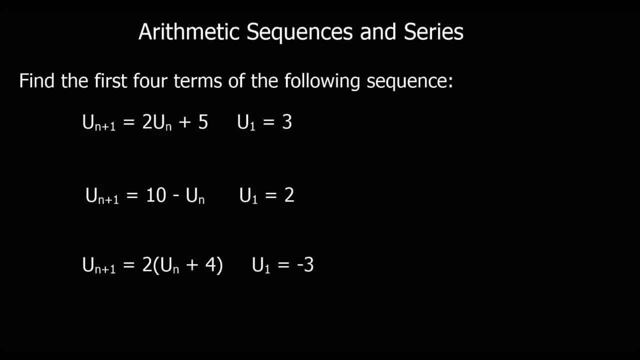 first term. get the answer. Substitute in the second term to find the third term. Substitute in the third term to find the fourth term. Okay, so to find the second term, I'm gonna do two, lots of the first term plus five, So the second term. 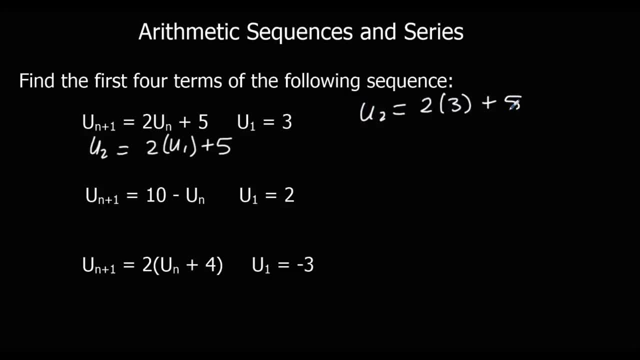 is gonna be two threes plus five. six plus five is 11.. Then to find the third term, that'll be two 11's plus five, which is 22 plus five is 27.. And to find the fourth term: two 27's plus five is 28.. You want to think about what we can do for an answer like that? 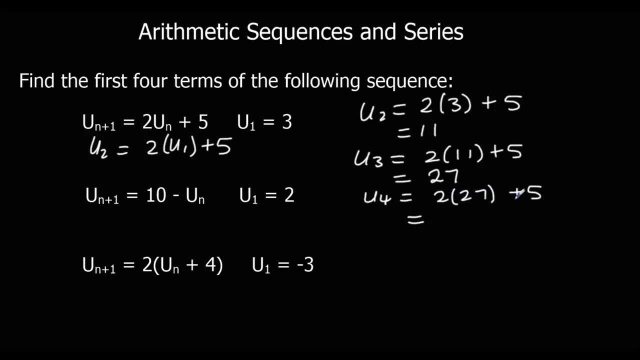 Okay, let's do this. two, lots of the first, third, So 1200 plus five, in plus nine and so on five, so that's 54 plus 5, which is 59. okay, the same for the second one, so the. 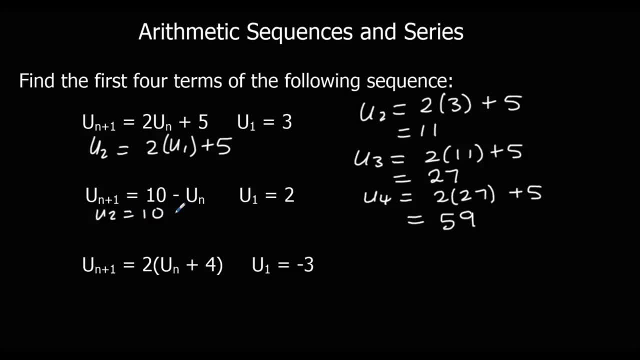 second term is 10 minus the first term. so if I do this one in red so we don't get confused, the second term read: so: the second one is 10, take away 2, which is 8. the third term is 10, take away 8, which is 2, and the fourth term will be ten. take, 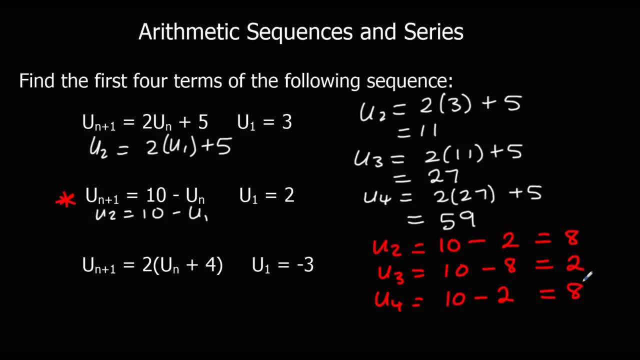 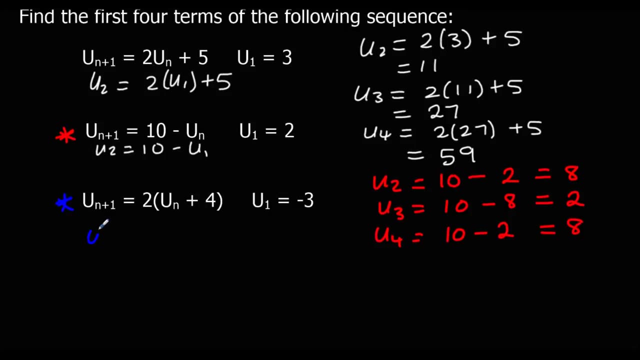 away two, which will be eight. so this progression is just going to keep going: eight, two, eight, two, eight, eight, eight, two, eight, two, 2, and so on, and finally the third one. so we'll do this. one in blue, this is saying so. the second term will be 2, lots of the first term plus 4. so we're gonna plus 4. 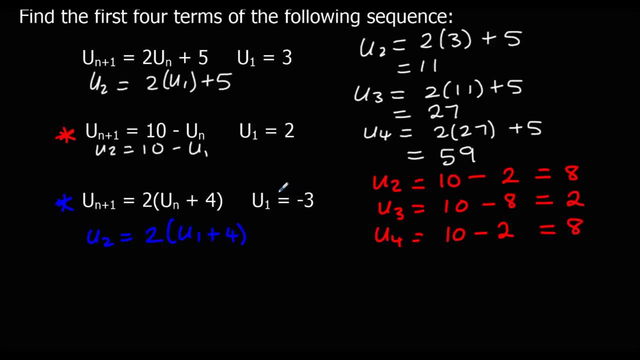 onto the first term and then multiply it by 2, so the first term is minus 3. so the second one is going to be 2 times minus 3 plus 4, which is 1. so the second term is 2 and the third term it's going to be 2, lots of 2 plus 4, which is 2 times 6. 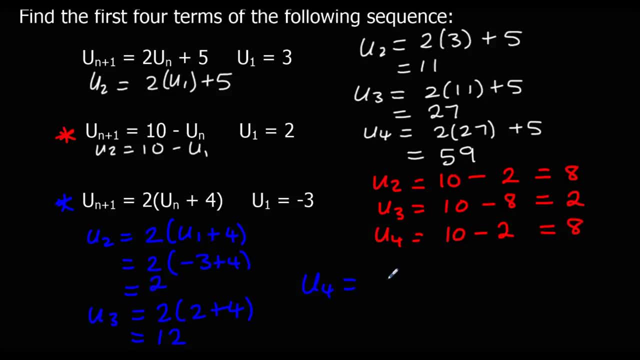 which is 12, and the fourth term will be 2, lots of 12 plus 4, so 16 times 2, 32 you. 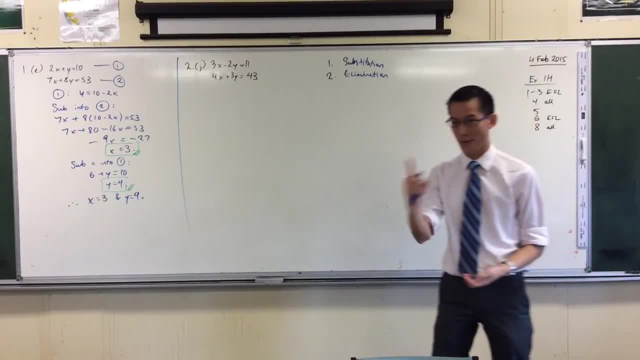 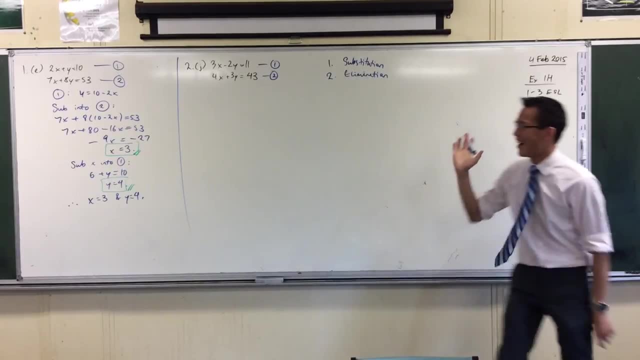 What shall I do here? What's my very, very, very first step? Thank you, well done. Ten points to Gryffindor. Okay, now, always do that, never just like before, when we were noticing when you're solving equations. 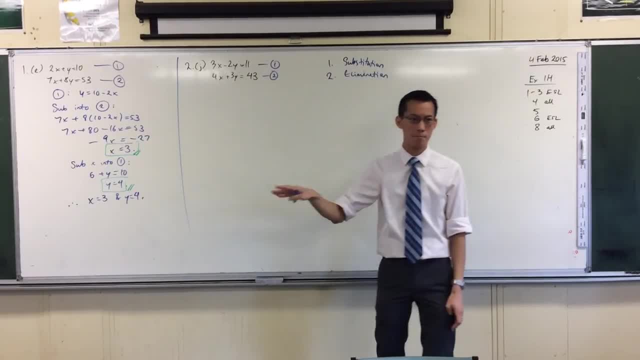 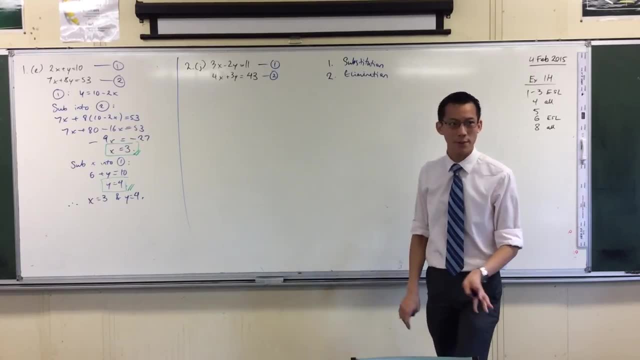 before you even start working. before you start working, you note restrictions or you draw a diagram, all those kinds of things with simultaneous equations. labelling them is exactly the same. Okay, before you go anywhere, Alright now if I'm doing this by elimination and you notice, by the way, I couldn't do this by substitution. 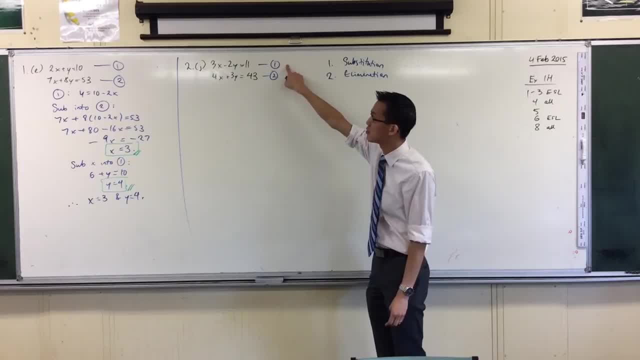 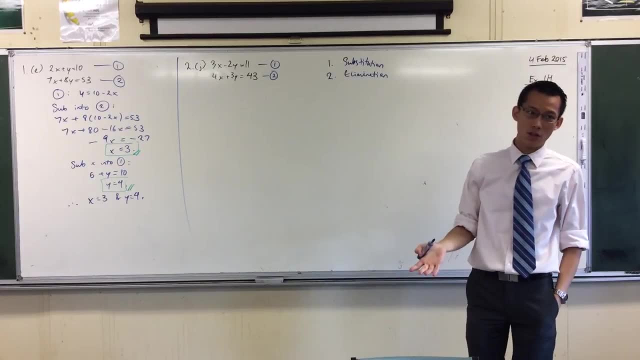 I suppose I would maybe divide this equation by two, this equation by three or etc. so that I can isolate one of the variables. But being that this time I've chosen to do it by elimination, I have two choices. I can multiply two different things.